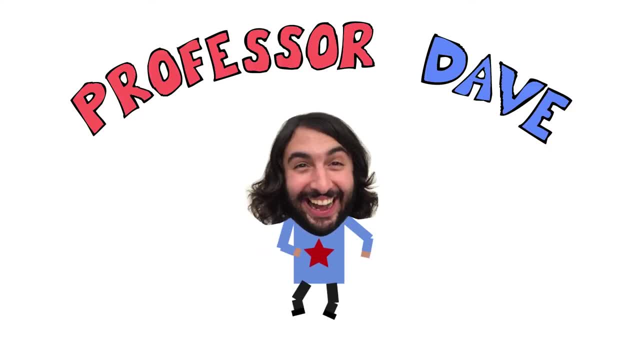 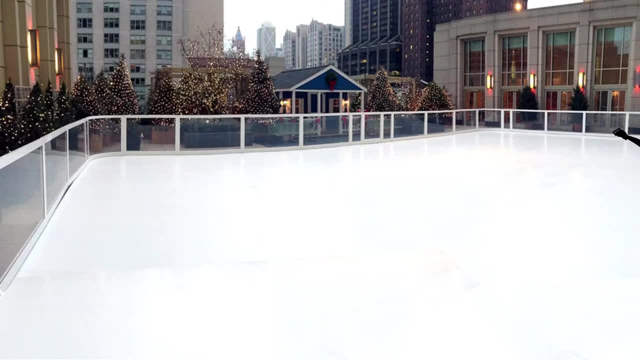 You and your friend decide to spend the afternoon at the ice skating rink. But to mix things up, you decide to bring a 0.2 kilogram frisbee. Much to the irritation of the other patrons at the rink, you begin to toss the frisbee. 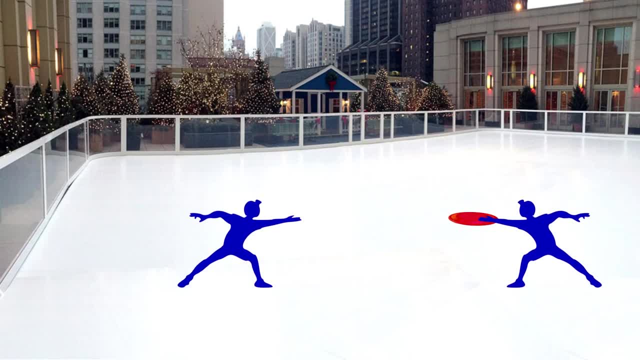 back and forth as you skate around. Given that you are both really into physics, right now you try an experiment. You stand perfectly still while your friend tosses you the frisbee as hard as they can, which turns out to be twenty meters per second. 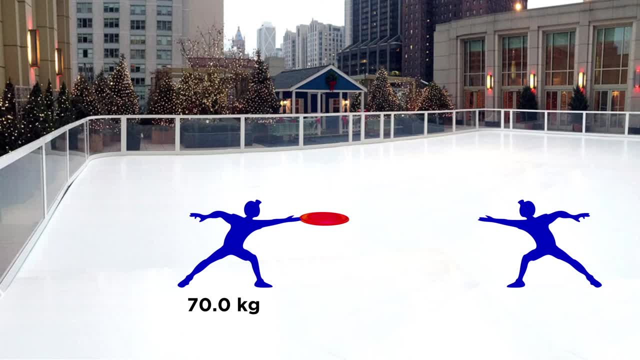 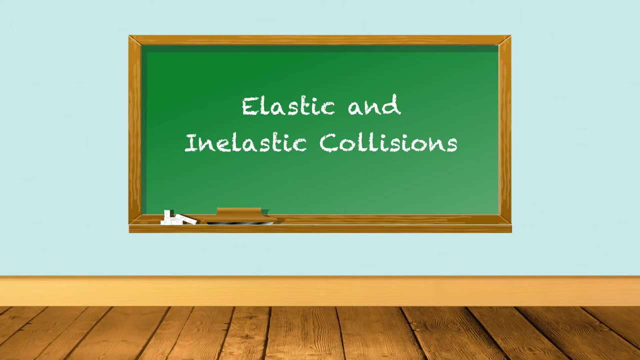 When you catch the frisbee, assuming the ice is frictionless, you and your seventy kilograms of mass are propelled backwards, but with what velocity? To figure this out, we just need equations regarding collisions, since we can consider catching a frisbee a collision. 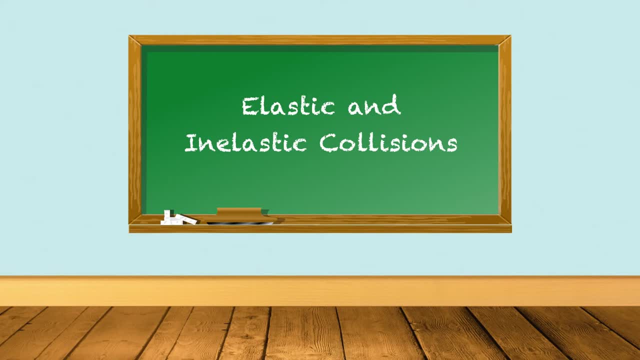 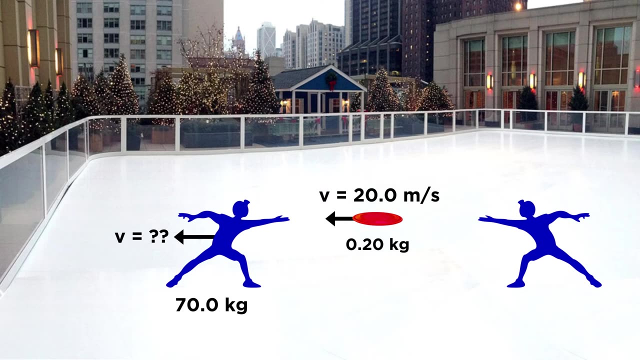 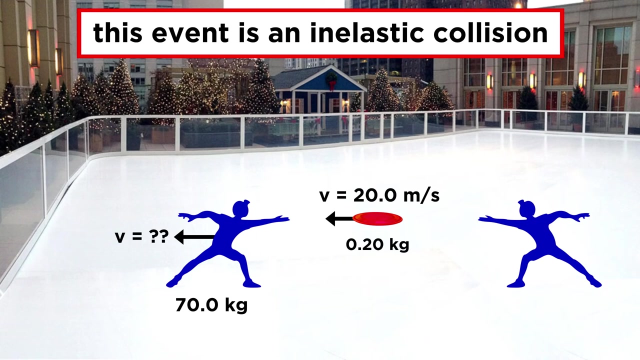 A collision of sorts. Check out my tutorial on this subject, if you need to, and then see what you come up with. Like I said, when you catch the frisbee, we can regard this as a collision, and, more specifically, an inelastic collision, as the frisbee doesn't bounce off of you, but rather you and the. 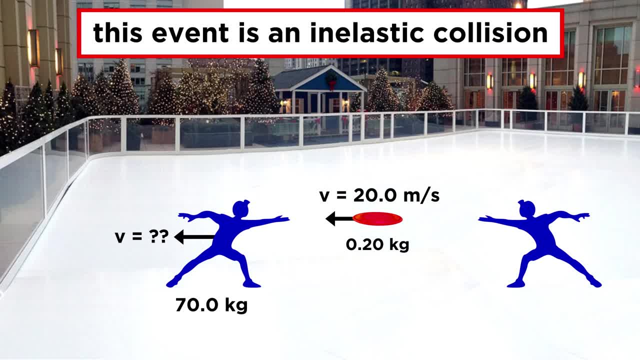 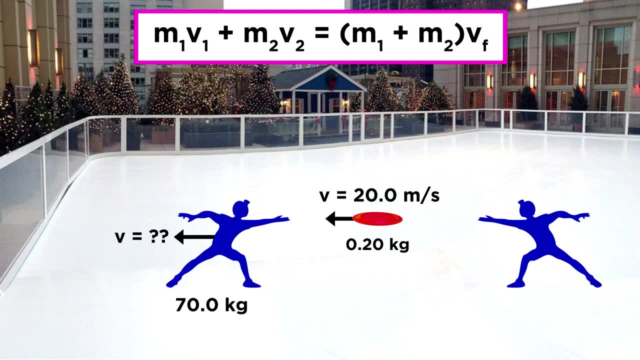 frisbee become one object moving together. The equation regarding inelastic collisions tells us that M1V1 plus M2V2 equals the quantity M1 plus M2 times V final. So let's just plug in everything we know. Taking you to be object one, your initial velocity was zero, so we can just get rid. 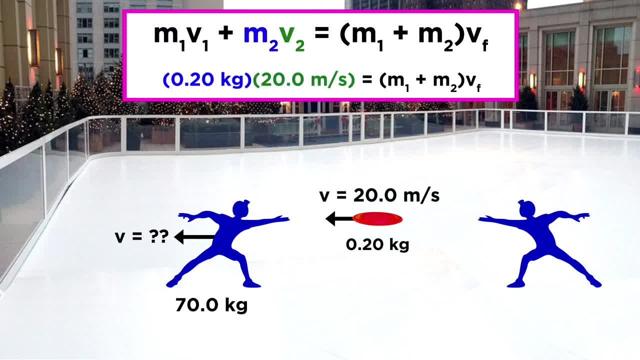 of this term. The frisbee has a mass of 0.2 kilograms and was moving at a speed of 20 meters per second. Then over here we can add the two masses to get 70.2 kilograms and then solve for. 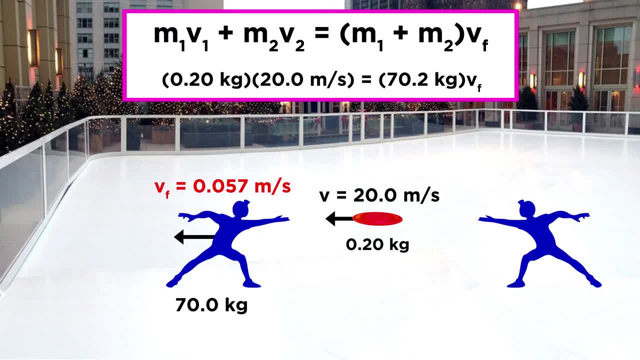 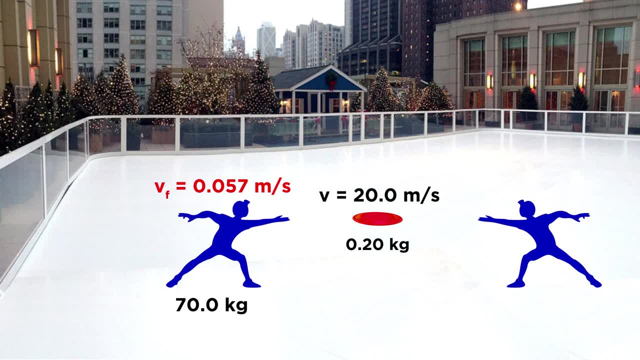 the final velocity That will give us 0.057 meters per second. This is pretty small, of course, given the huge difference in mass between you and the frisbee, but it's still a pretty interesting way to get across the ice.